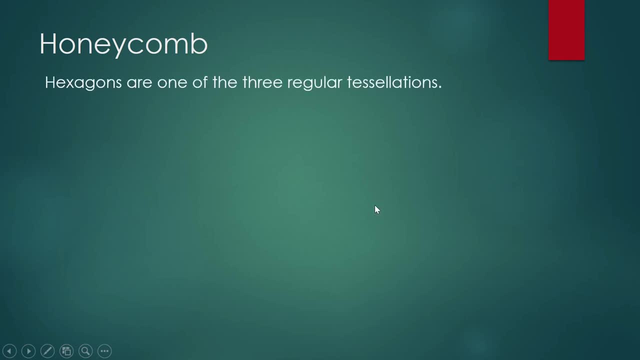 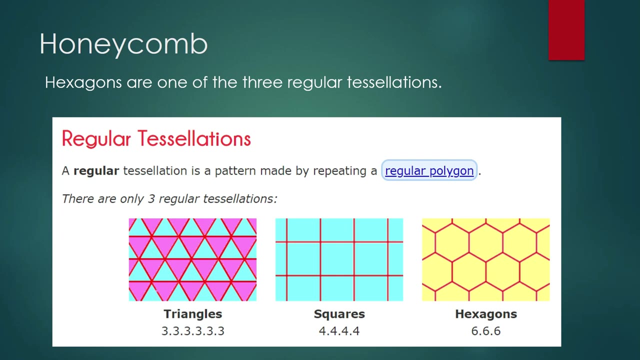 made from tiny hexagons is fascinating enough that they had the attention of mathematicians ever since the days of the ancient Greeks. What is fascinating about hexagons is hexagon is one of the three regular polygon which you can use to produce a regular tessellation. A tessellation is: 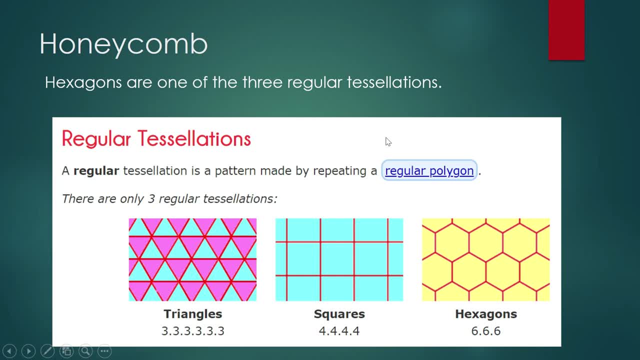 something like this: You have: you have a plane and you want to cover it with polygons. But you want to cover it with polygons in such a way that the polygons will not overlap and there will be no gaps between the polygon And there are three polygons or regular polygons that can do that. 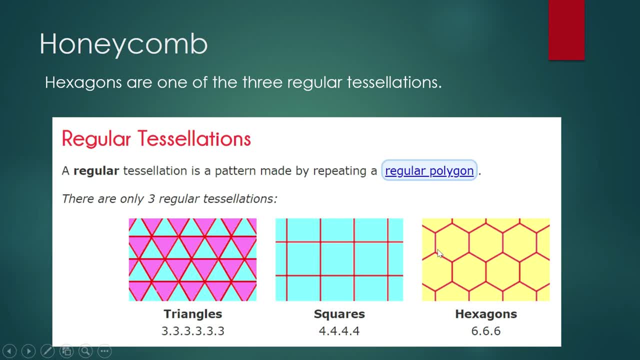 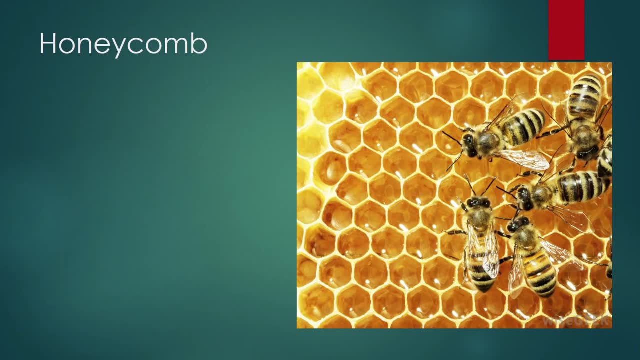 That would be the triangles, the squares, and one of them would be the hexagons, And honeycombs are constructed using regular hexagons. There was one mathematician who is so fascinated by this and he made this. He made this comment: Bees must be imbued with natural wisdom, because they knew that hexagon is. 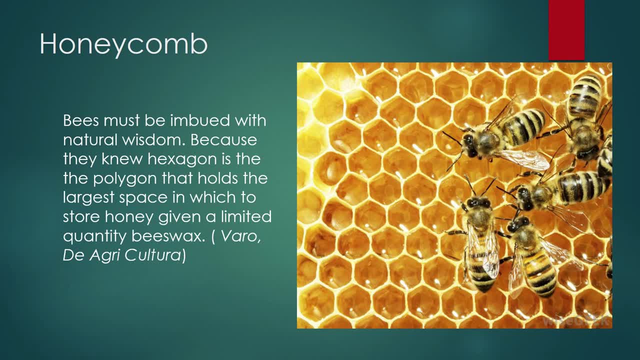 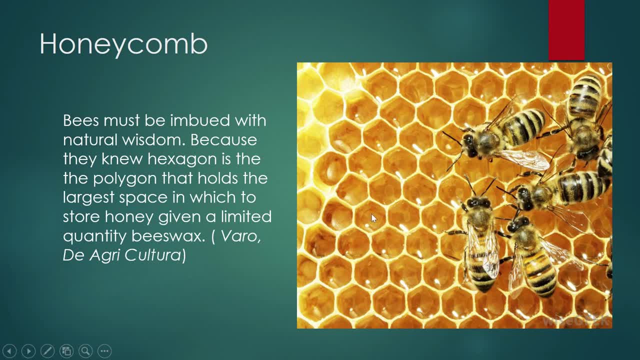 compartmentalized honeycombs. What would be the best shape of the compartment, or what will be the best shape of the holes, such that it can hold the largest quantity of honey? That kind of problem abound in applied math, and we call it optimization. 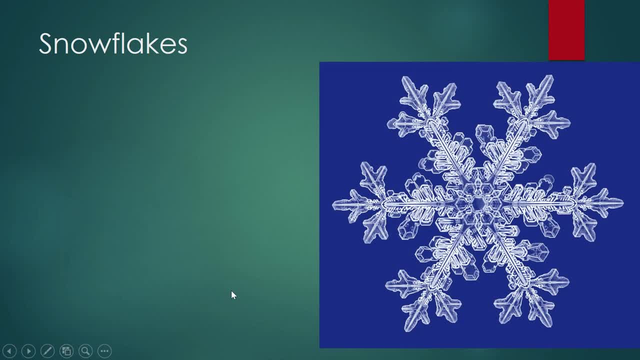 Snowflakes. I have not seen a snowflake in my life, So these are icicles. So these are small eyes formed around suspended dusts and they show self-repeating patterns. So snowflakes show this thing which we call fractals. 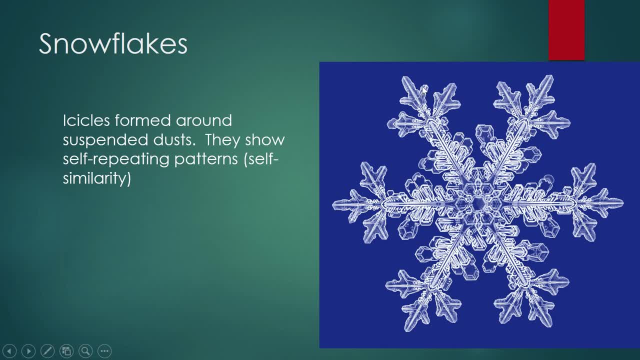 They show self-repeating patterns When you look at the small parts of it. the small parts seem to be a tiny reproduction of the bigger parts of the snowflake Fractals. This is what I said earlier. Fractals are objects whose smaller parts look similar to the larger parts of the object. 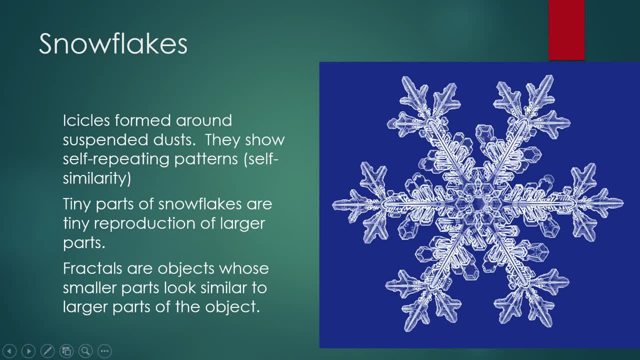 I have not seen icicles in my life, but what I had seen are balls of ice. I experienced seeing balls of ice falling from the sky and I thought, hey, are we in the United States now? Are we in Canada now? 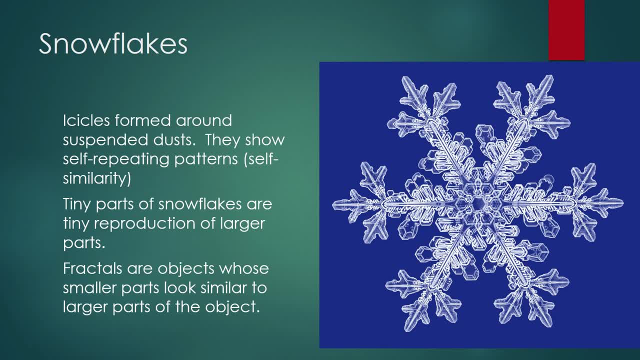 But we are not in those places. We are right here in Batangas. When I was a kid, I experienced balls, Balls of ice falling from the sky, and it was not an amusing experience. Well, the initial thought of it is kind of amusing. 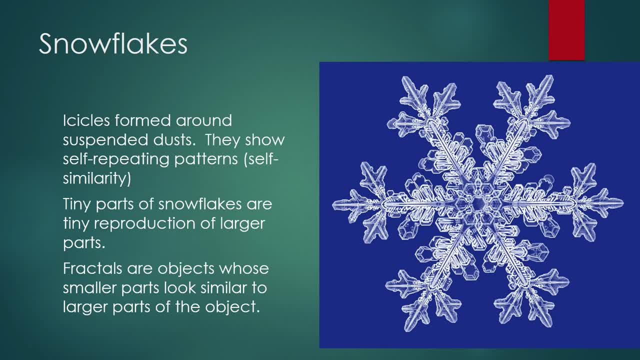 but when we saw the size of the ice, they were as big as golf balls. They are no longer amusing when balls like that can hurt you. So again, fractals are objects whose smaller parts look similar to the larger parts of the object. 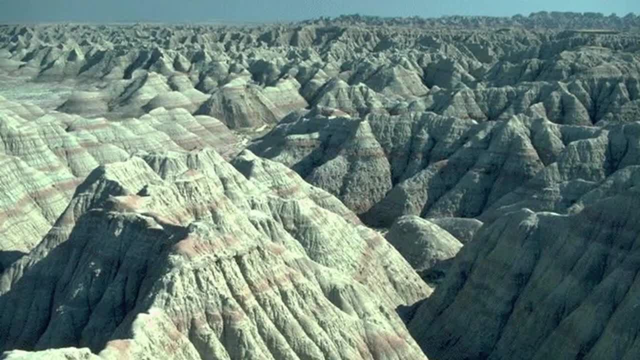 And that is precisely the experience that we see when we look at a mountain. Okay, You know what? When I was a kid, I liked to play with toy soldiers, Toy soldiers, and so in my mind, the soldiers will hide in the mountain. 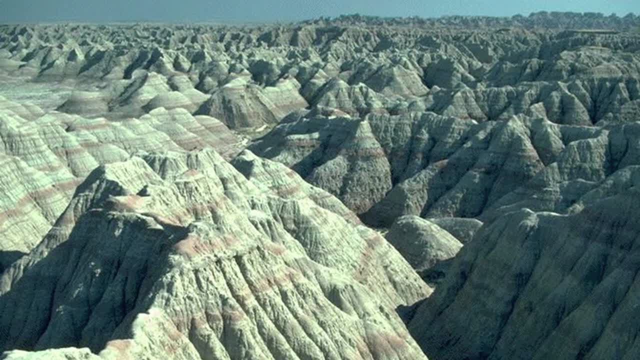 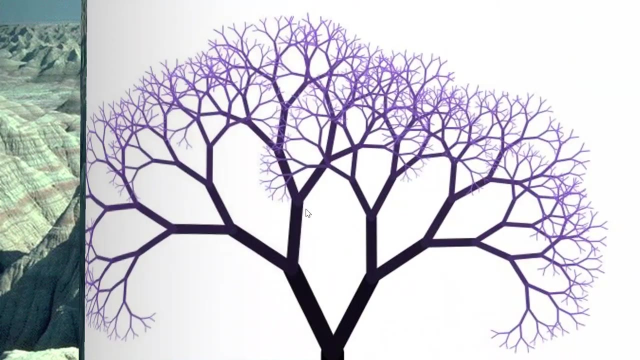 but the mountain is just a mound of soil. But when you look at that mound from afar or even closer, they in fact look like something like this: They look like mountains. So mountains show the phenomenon of fractals of self-similarity. 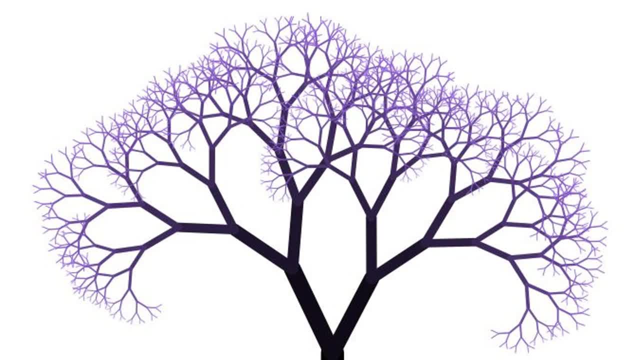 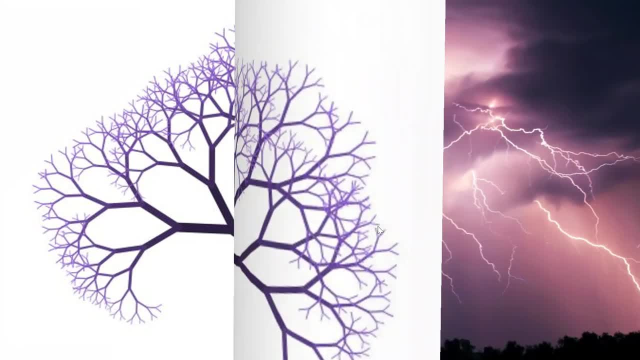 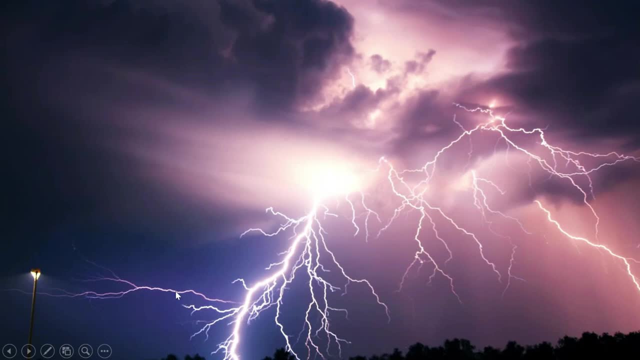 trees also show the phenomenon of self-similarity. When you look at one branch, it is a reproduction of the other branches in the tree. The same with lightning. Look at one arm of the lightning. In fact, each arm of the lightning seems to be a reproduction of the other arms or branches of the lightning.